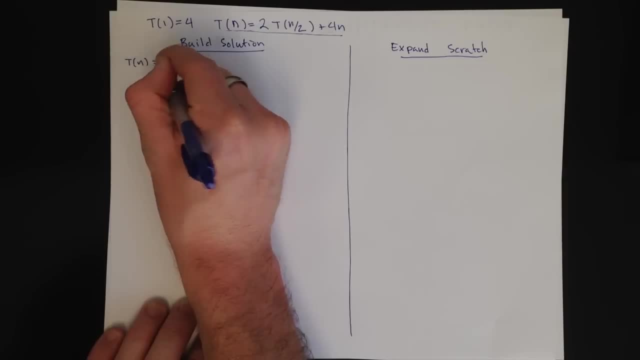 So we're going to start building a solution here, For t of n is equal to, and right now the best thing we know is that t of n is equal to 2t of n over 2 plus 4n, And what can I apply here? 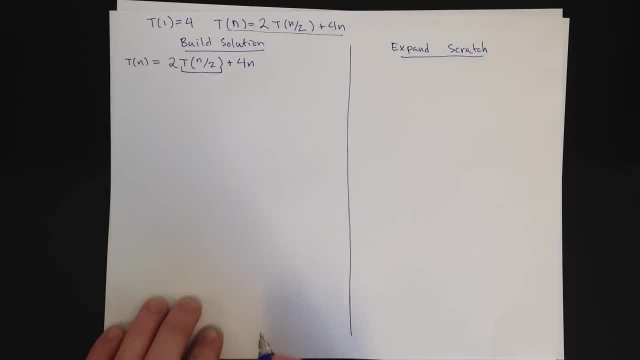 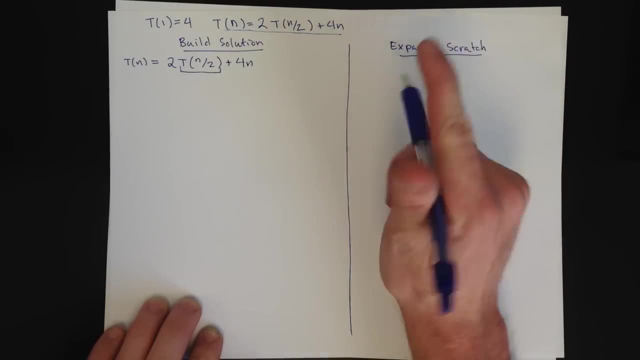 The only thing I can do is expand t of n over 2 and then plug it back in. This is why this is often called the plug and chug. So now I need to do an expansion. I'm going to do it on my scratch pad. 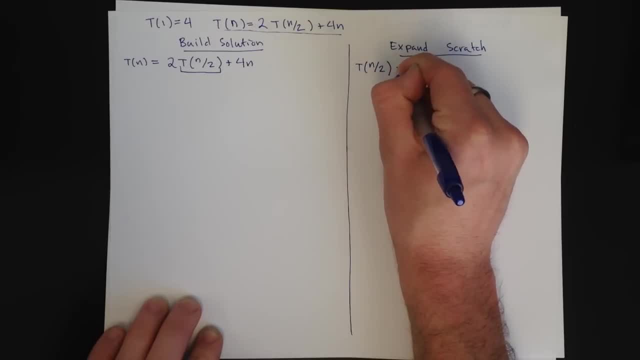 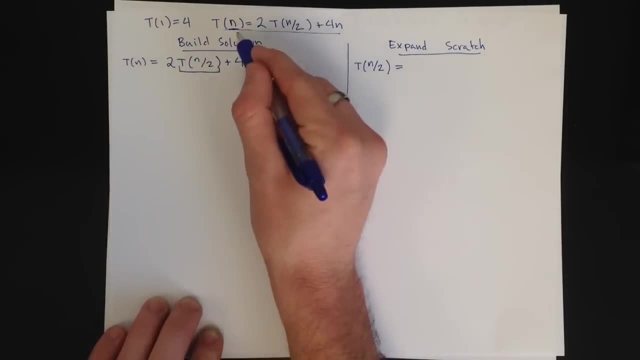 And over here I write t of n over 2.. And the question is: what is this equal to? Well, I know how to plug something in for t Here. I called it n. What I'm plugging in is the n over 2.. 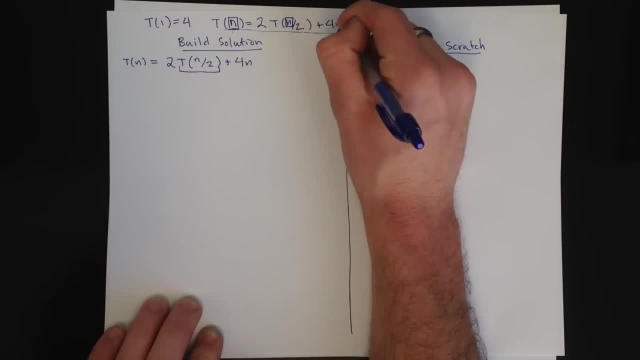 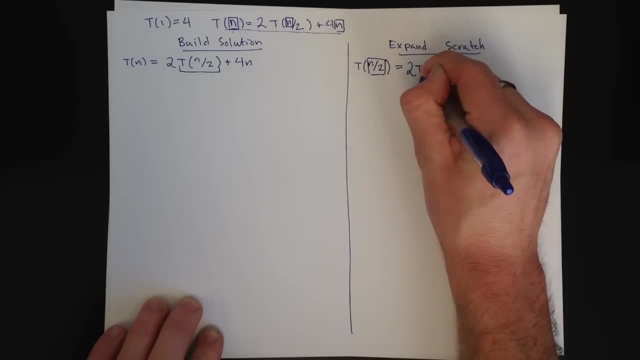 Plugging it in for n, which means that anywhere I see n, I need to replace it with t of n over 2.. So I get 2t of, and now I had n over 2 before, but now I'm plugging in n over 2 itself. 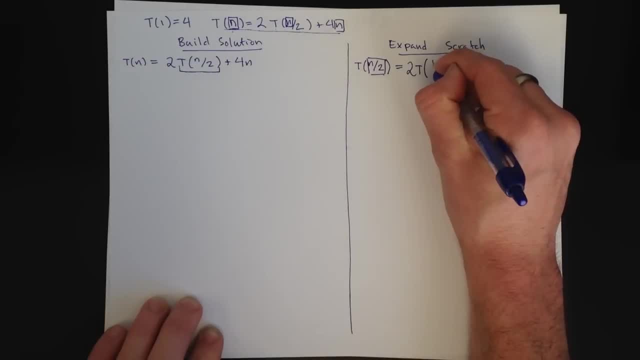 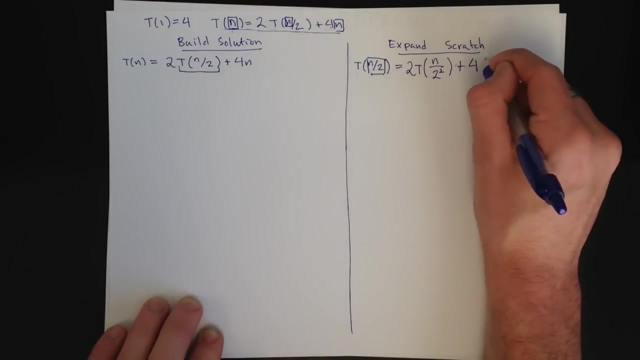 So this is n over 2 over 2, which is n over 2.. n over 2 squared. And then I need to add the rest plus 4 times what was in here. So if it were n, I'd put n, but here I have n over 2, so I'm plugging in n over 2, and I get this. 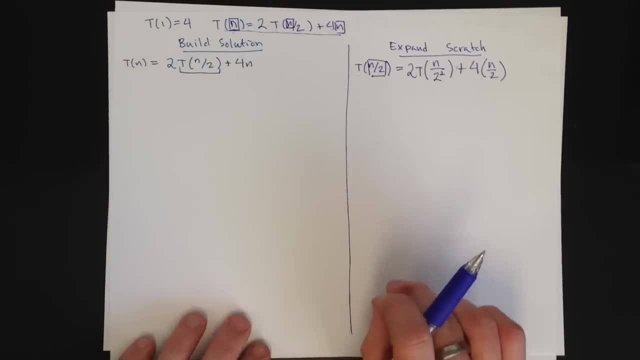 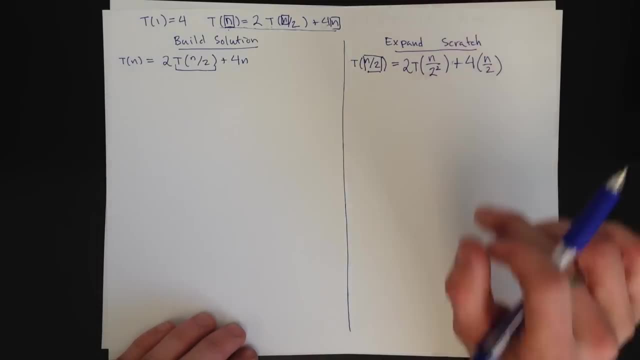 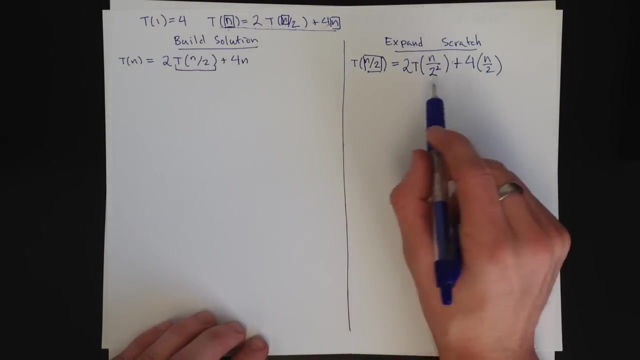 Now one thing to keep in mind: I could write 2 squared here as 4, and I could write 4n over 2 as 2n instead of leaving it like this. But often I find I find it easier with the substitution method to figure out the pattern if I leave things a little bit unsimplified. 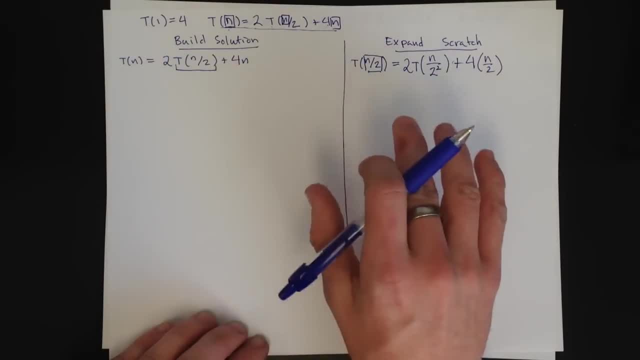 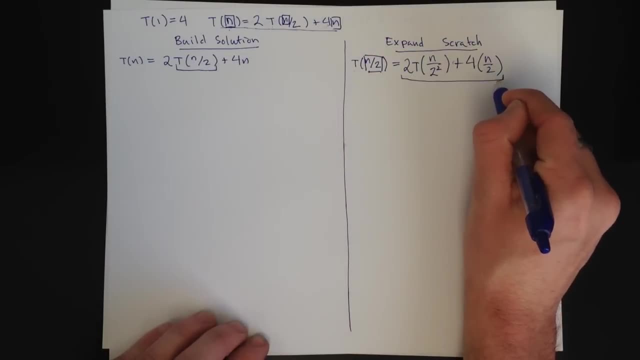 And so that's the way I'm going to leave it. I'm going to leave it exactly like this, And now what I need to do is take: I have t of n over 2. here I've figured out something that t of n over 2 is equal to by doing an expansion. 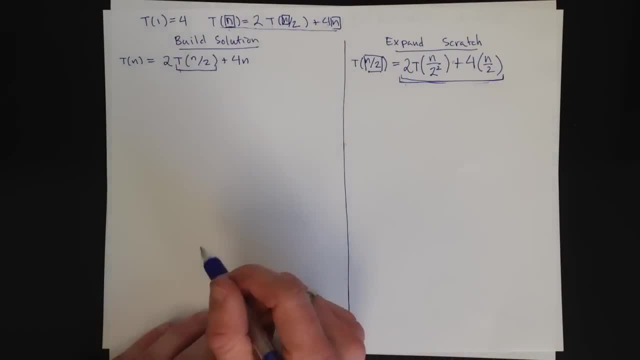 and so I need to plug into this equation this value. So, to do it really carefully, what I usually do is say equals 2, and then, And for where I'm going to plug this in, add a whole bunch of space, enough space to stick this thing inside it. 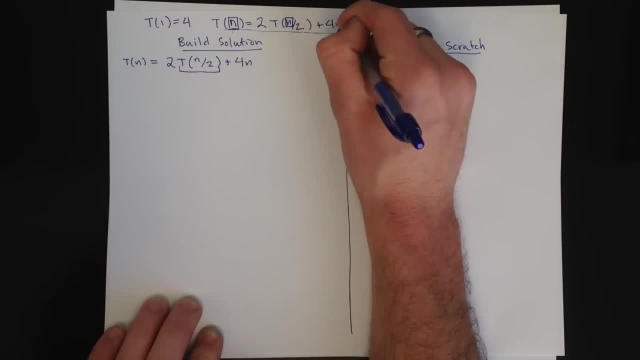 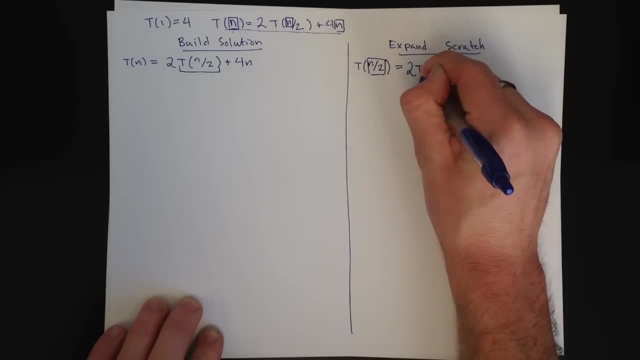 Plugging it in for n, which means that anywhere I see n, I need to replace it with t of n over 2.. So I get 2t of, and now I had n over 2 before, but now I'm plugging in n over 2 itself. 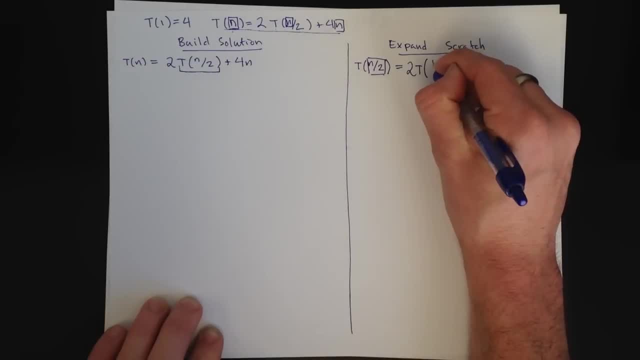 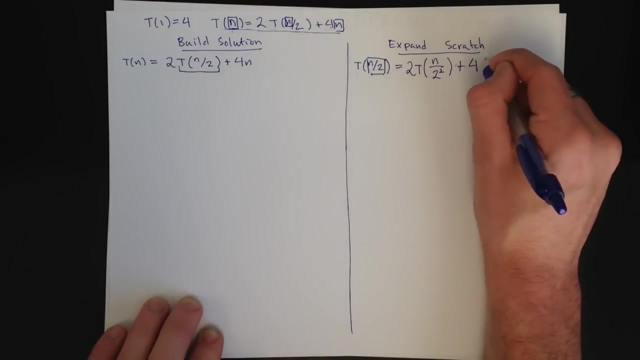 So this is n over 2 over 2, which is n over 2.. n over 2 squared. And then I need to add the rest plus 4 times what was in here. So if it were n, I'd put n, but here I have n over 2, so I'm plugging in n over 2, and I get this. 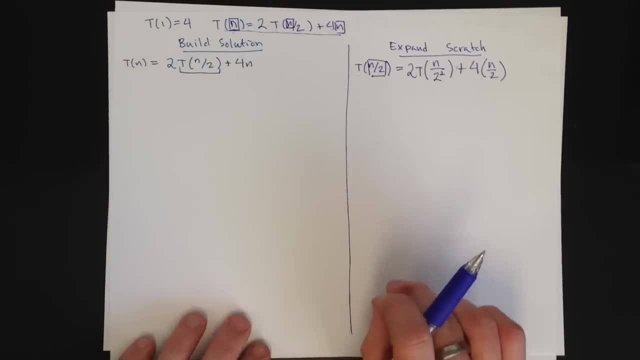 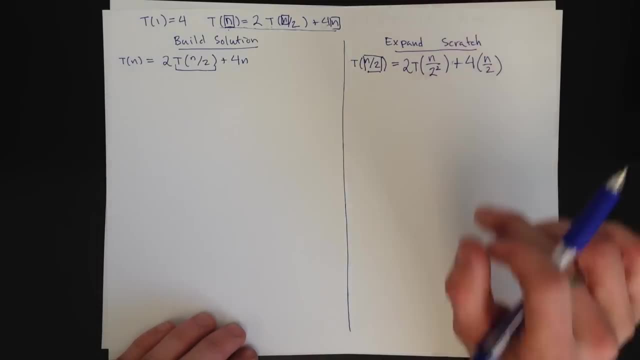 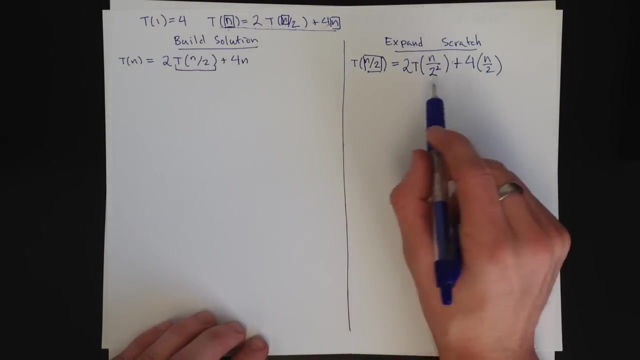 Now one thing to keep in mind: I could write 2 squared here as 4, and I could write 4n over 2 as 2n instead of leaving it like this. But often I find I find it easier with the substitution method to figure out the pattern if I leave things a little bit unsimplified. 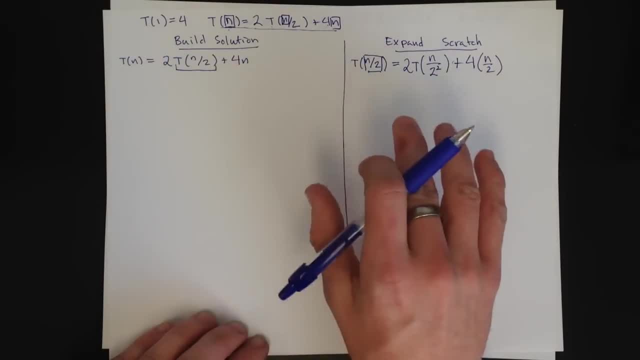 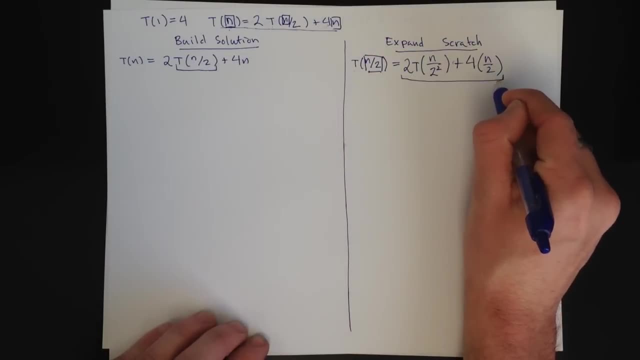 And so that's the way I'm going to leave it. I'm going to leave it exactly like this, And now what I need to do is take: I have t of n over 2. here I've figured out something that t of n over 2 is equal to by doing an expansion. 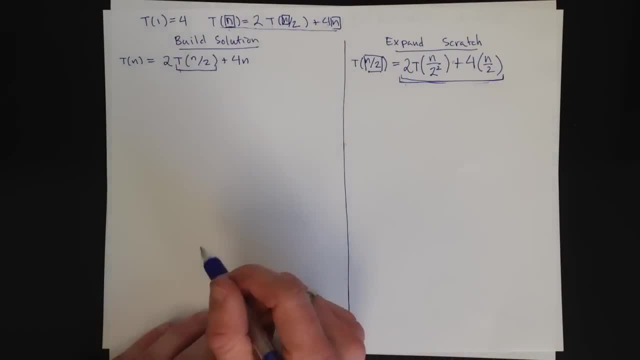 and so I need to plug into this equation this value. So, to do it really carefully, what I usually do is say equals 2, and then, And for where I'm going to plug this in, add a whole bunch of space, enough space to stick this thing inside it. 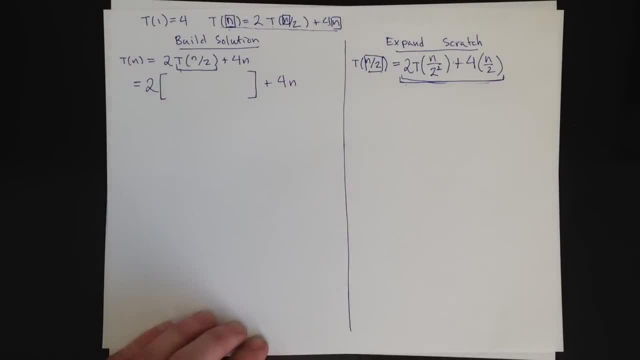 and then I have to write the rest of my equation plus 4n. So far, so good. Now what goes in here is exactly this: 2t of n over 2, squared plus 4n over 2.. And then the next step is to go ahead and multiply through. 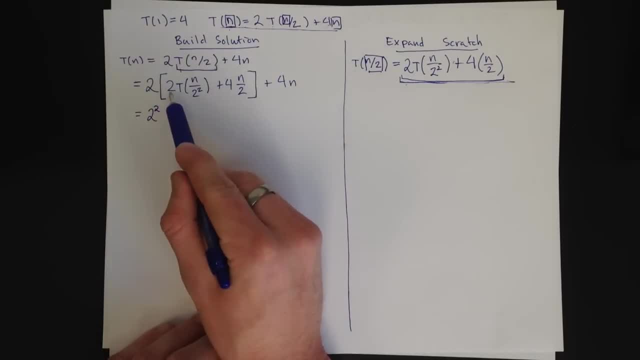 So this becomes 2 squared. By the way, I also like keeping things In terms of powers, because I keep repeating these operations so things tend to turn into powers. So instead of saying 4, it's better to say 2 squared. 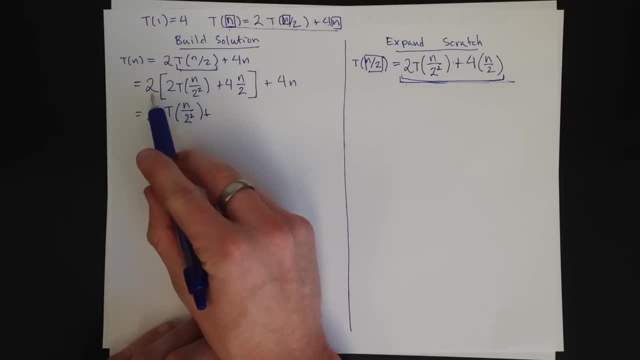 2 squared plus. And now notice, when I multiply this 2 times 4n over 2, the 2s cancel. So I just get 4n plus 4n. All right Now, what can we do? The only thing we can do is expand. 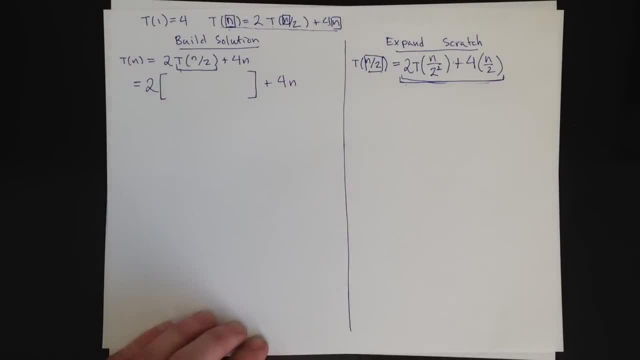 and then I have to write the rest of my equation plus 4n. So far, so good. Now what goes in here is exactly this: 2t of n over 2, squared plus 4n over 2.. And then the next step is to go ahead and multiply through. 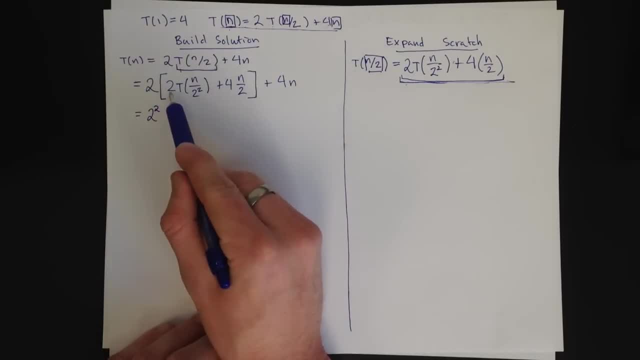 So this becomes 2 squared. By the way, I also like keeping things In terms of powers, because I keep repeating these operations so things tend to turn into powers. So instead of saying 4, it's better to say 2 squared. 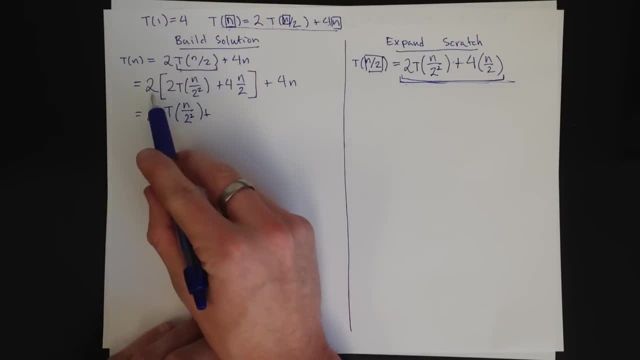 2 squared plus. And now notice, when I multiply this 2 times 4n over 2, the 2s cancel. So I just get 4n plus 4n. All right Now, what can we do? The only thing we can do is expand. 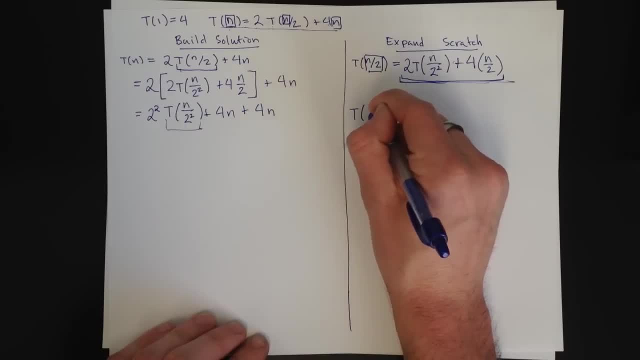 That's the only thing we know. We don't know how to do here, So we're going to expand again. This time we're expanding t of n over 2 squared. Plugging in n over 2 squared for n gives us 2t. 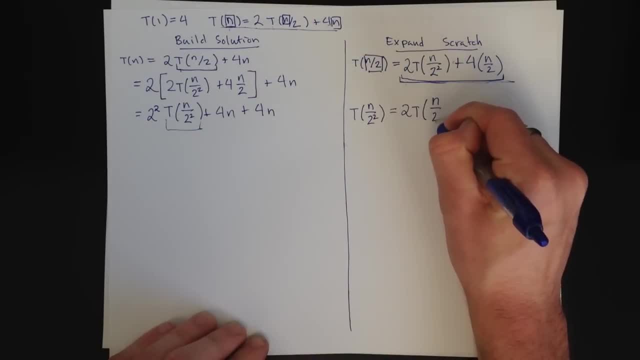 and n over 2 squared. divided by 2 is n over 2 cubed plus 4n over 2 squared. And now I need to plug this back in. What's this plug-in? chug 2 squared, create a big block. 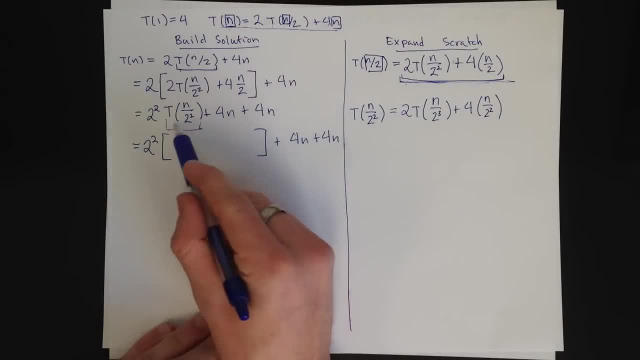 plus the 4n plus the 4n. So I'm just coming down, put this inside: t of n over 2 cubed plus 4n over 2 squared. Copied that over. All right, And now I multiply through. 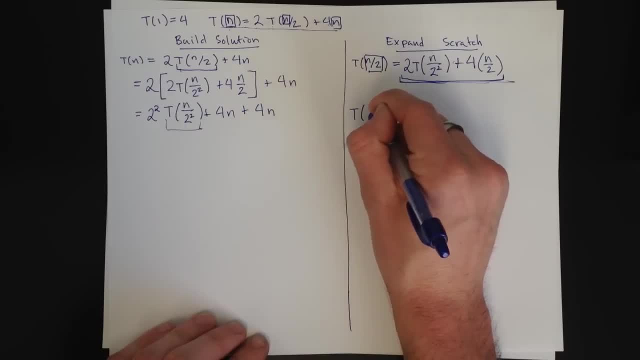 That's the only thing we know. We don't know how to do here, So we're going to expand again. This time we're expanding t of n over 2 squared. Plugging in n over 2 squared for n gives us 2t. 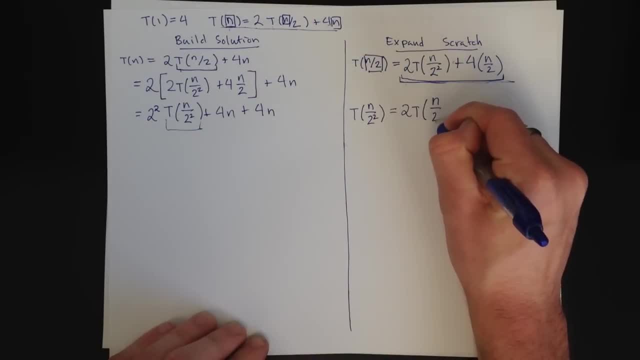 and n over 2 squared. divided by 2 is n over 2 cubed plus 4n over 2 squared. And now I need to plug this back in. What's this plug-in? chug 2 squared, create a big block. 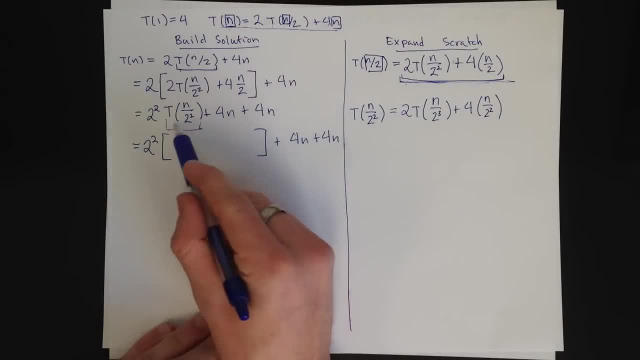 plus the 4n plus the 4n. So I'm just coming down, put this inside: t of n over 2 cubed plus 4n over 2 squared. Copied that over. All right, And now I multiply through. 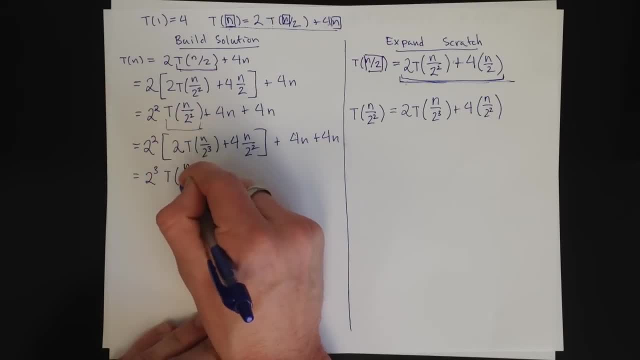 This becomes 2 cubed t of n over 2 cubed plus and the 2 squareds cancel. so I get a 4n and I had 2 of those already plus 4n. Hopefully you're starting to see a pattern here. 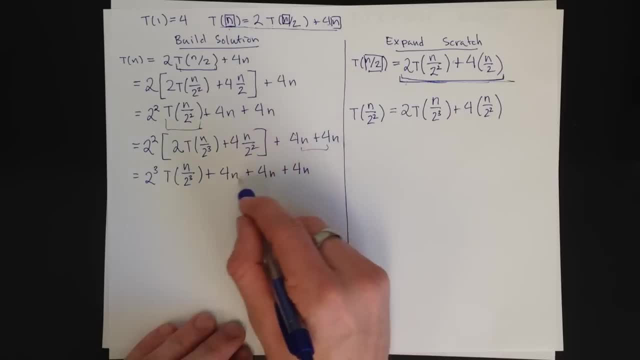 There are two 4n's here. There are three 4n's here. I'm raising things to squares up here- Sorry I shouldn't be doing this one And cubes down here, But we want you to do this three times. 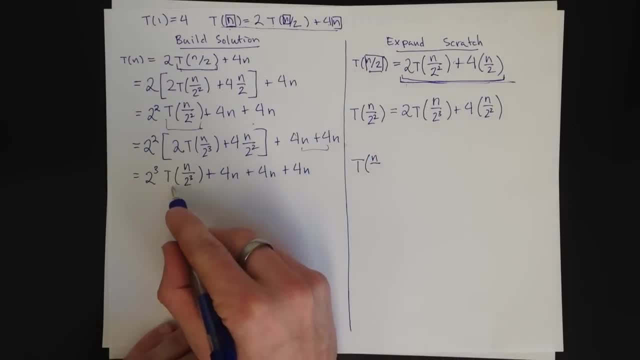 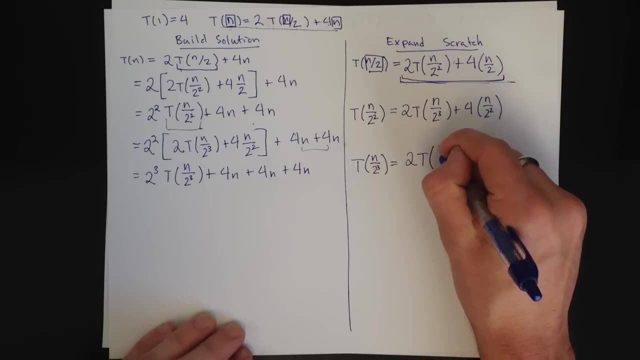 so you really make sure you see the pattern. So let's do it one more time. Now we need to plug in n over 2 cubed. This becomes 2t. Plugging in n over 2 cubed gives us n over 2 to the 4th. 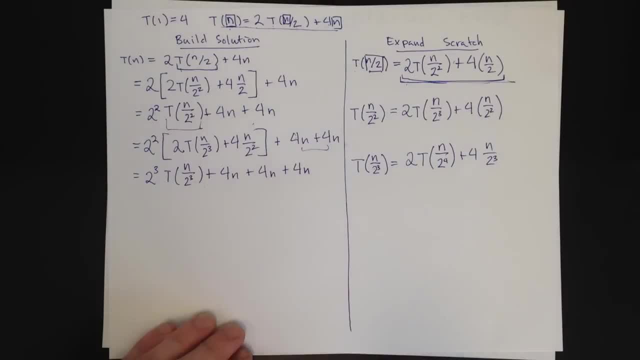 plus 4n over 2 cubed. Plug this in, We get 2 cubed. Create a big block for what I'm plugging in- the t of n over 2 cubed and then go ahead and write the rest of the line. 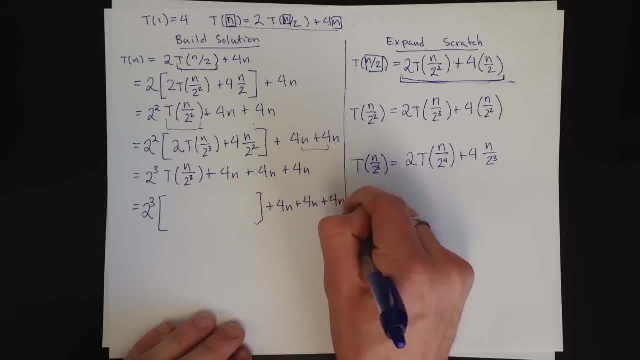 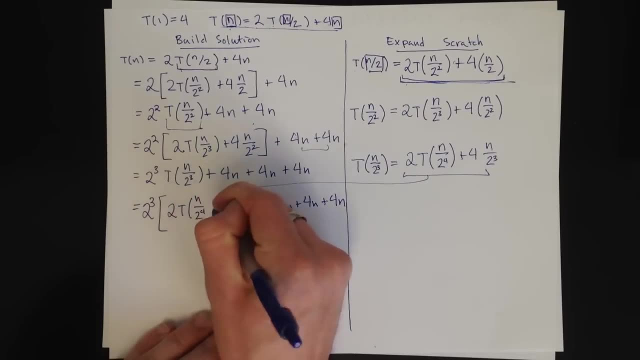 so I don't get confused later. And then plug that into there: 2t of n over 2 to the 4th plus 4n over 2 cubed, And then plug that into there. And then plug that into there. 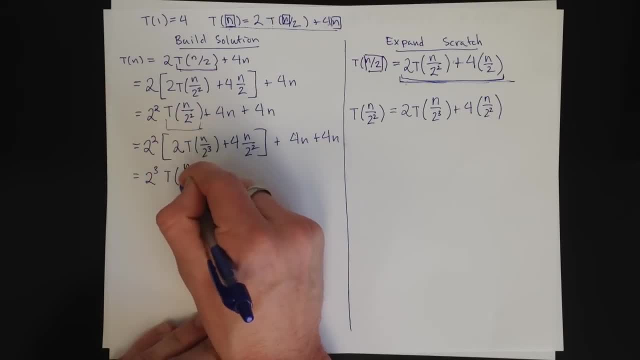 This becomes 2 cubed t of n over 2 cubed plus and the 2 squareds cancel. so I get a 4n and I had 2 of those already plus 4n. Hopefully you're starting to see a pattern here. 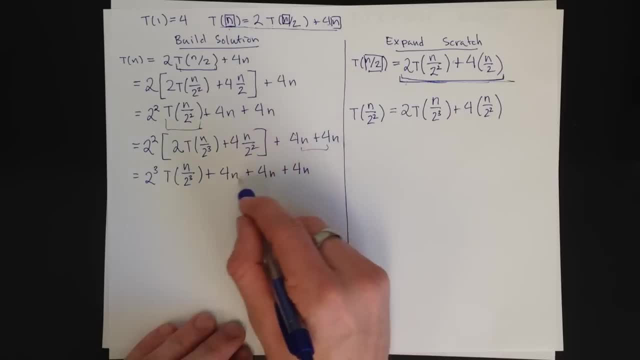 There are two 4n's here. There are three 4n's here. I'm raising things to squares up here- Sorry I shouldn't be doing this one And cubes down here, But we want you to do this three times. 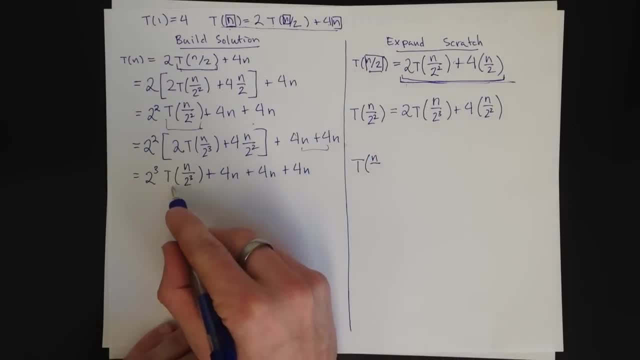 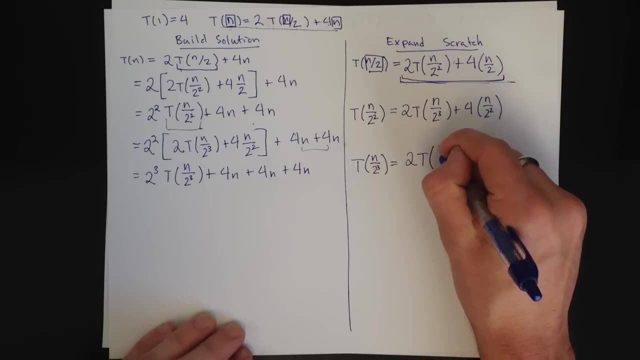 so you really make sure you see the pattern. So let's do it one more time. Now we need to plug in n over 2 cubed. This becomes 2t. Plugging in n over 2 cubed gives us n over 2 to the 4th. 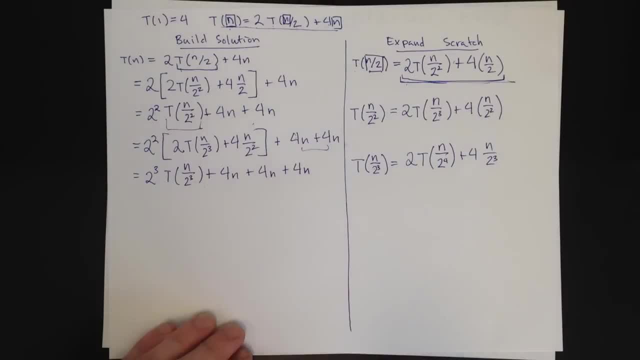 plus 4n over 2 cubed. Plug this in, We get 2 cubed. Create a big block for what I'm plugging in- the t of n over 2 cubed and then go ahead and write the rest of the line. 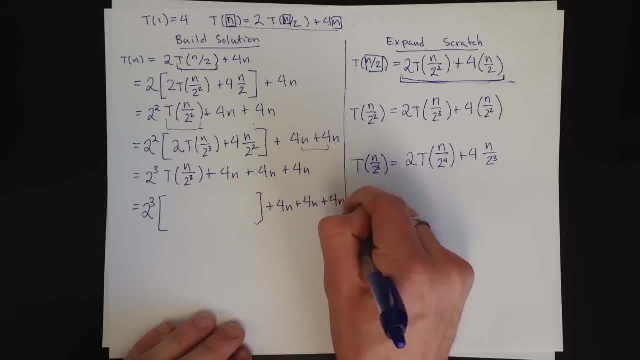 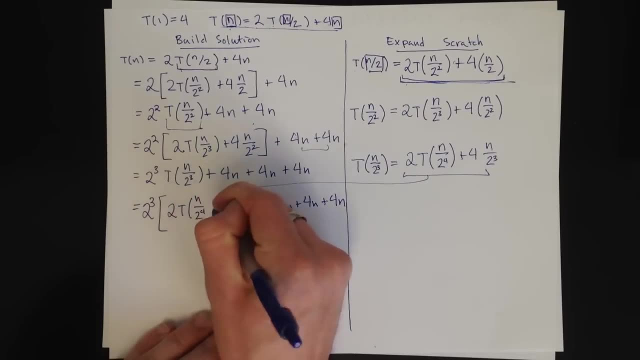 so I don't get confused later. And then plug that into there: 2t of n over 2 to the 4th plus 4n over 2 cubed. And then plug that into there 2t of n over 2 to the 4th. 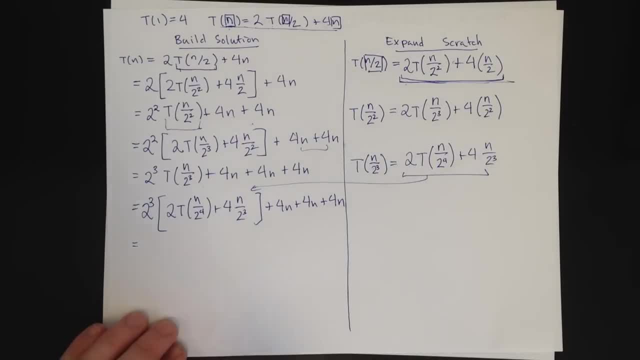 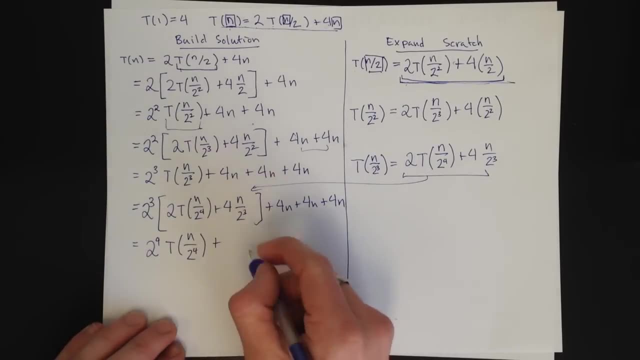 and multiply the 2 cubed through, So this becomes 2 to the 4th t of n over 2 to the 4th, plus the 2 cubes. cancel 4n plus 4, plus 4n plus 4n. 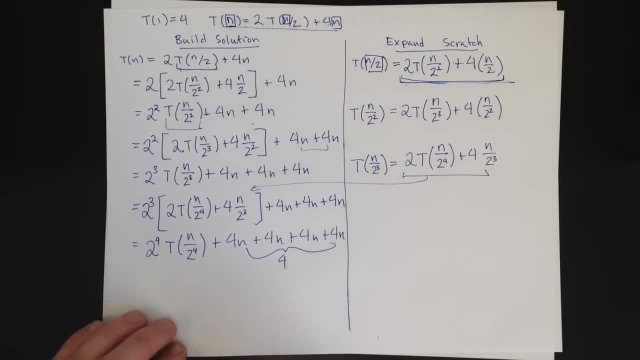 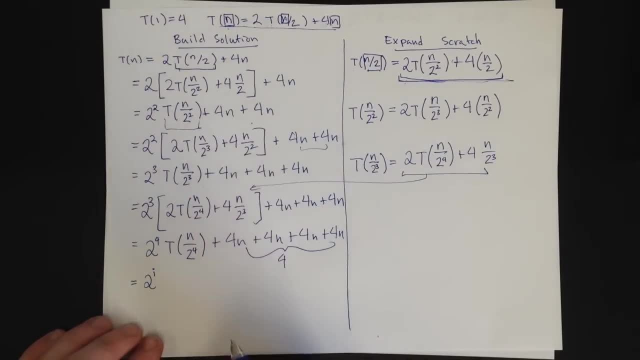 So there are 4 of these, And now it should be fairly easy to see the general case. Here. I have 2 to the i, based on how many times I've done this times t to the i and t to the n over 2i. 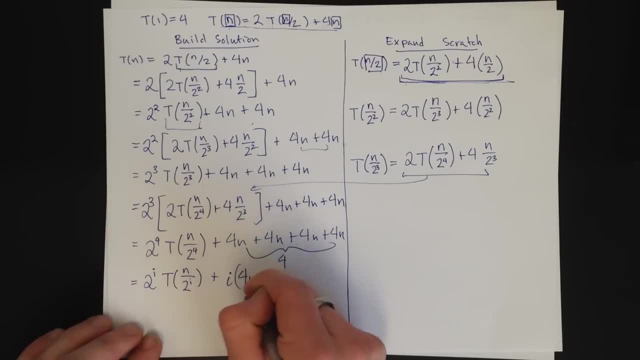 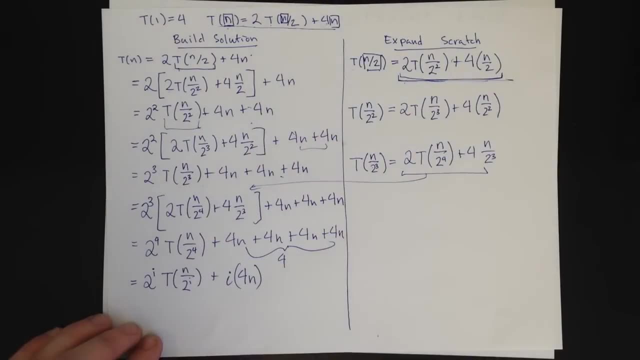 plus i times 4n, Because I had 4 times 4n here, I had 3 times 4n here, I had 2 times 4n here and 1 times 4n here. All right. Now the question is: 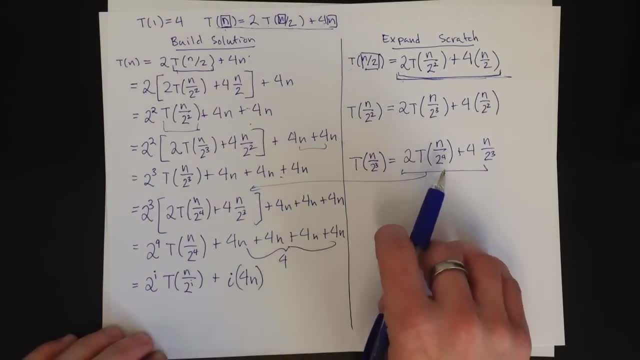 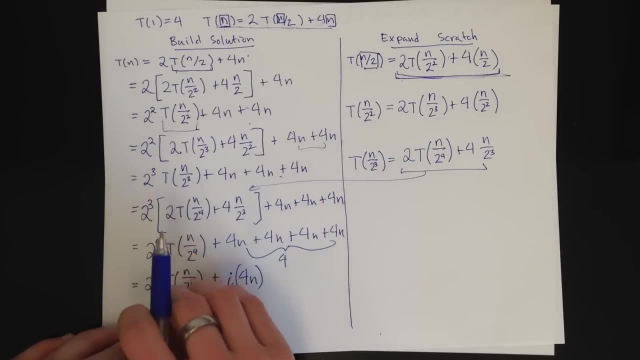 if I kept doing this process- bringing it the thing I need to expand out here, expanding it and plugging it back in- simplifying, bringing it out, expanding it, plugging it back in and simplifying- how many times would I do this? 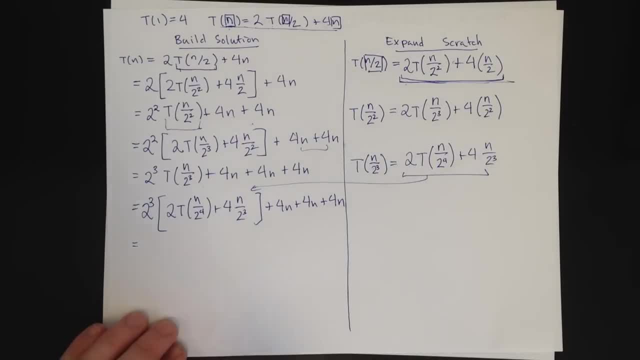 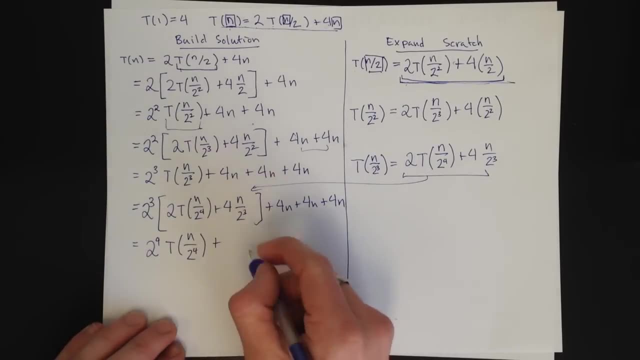 2 cubed and multiply the 2 cubed through, So this becomes 2 to the 4th t of n over 2 to the 4th plus the 2 cubes. cancel 4n plus 4, plus 4n plus 4n. 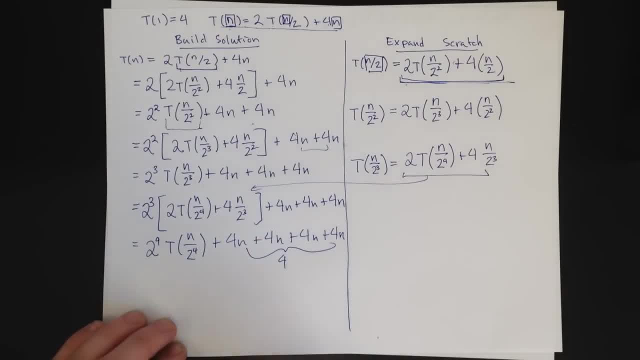 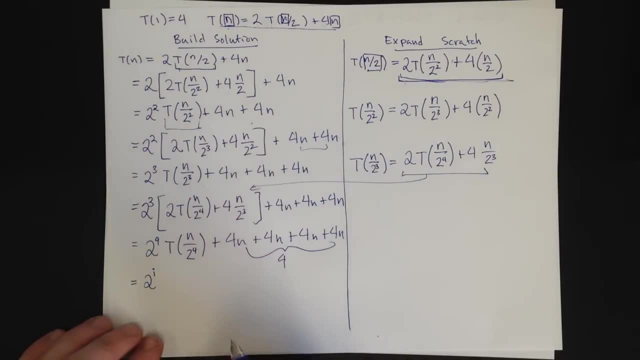 So there are 4 of these, And now it should be fairly easy to see the general case. Here. I have 2 to the i. based on how many times I've done this times t to the n over 2 cubed. 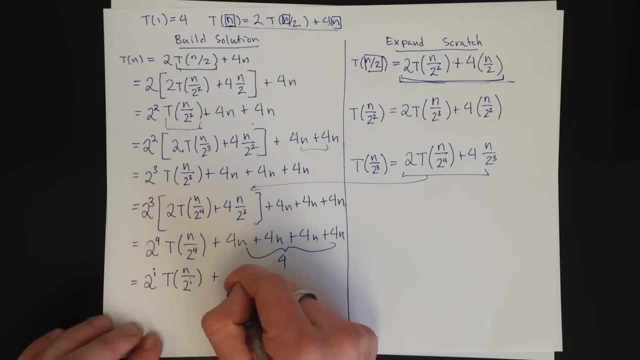 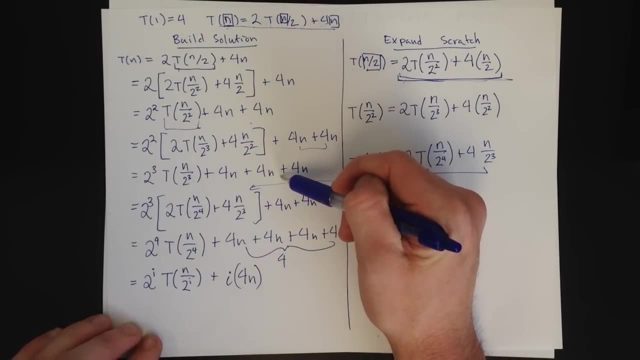 times t to the n over 2. i plus i times 4n, Because I had 4 times 4n here, I had 3 times 4n here, I had 2 times 4n here and 1 times 4n here. 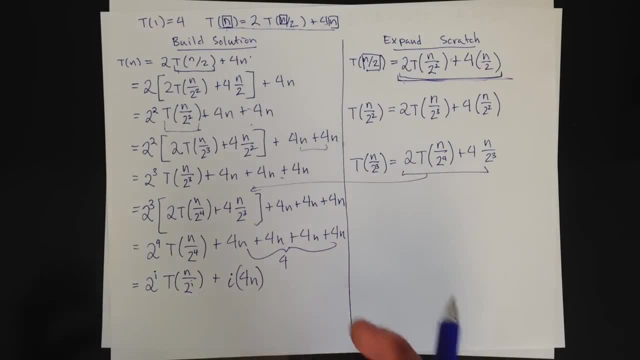 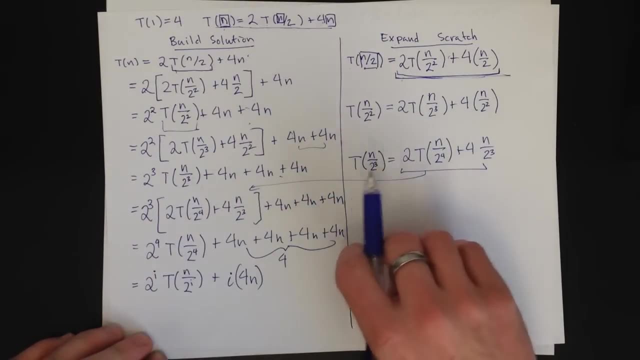 All right. Now the question is if I kept doing this process, bringing it the thing I need to expand out here, expanding it and plugging it back in. simplifying bringing it out, expanding it, plugging it back in. 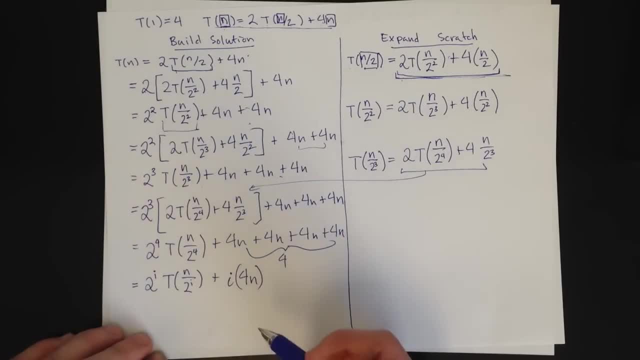 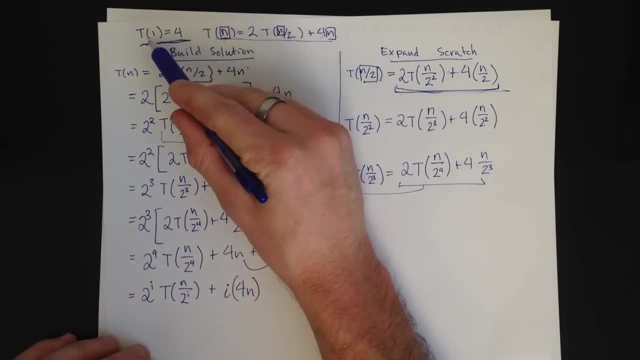 and simplifying. how many times would I do this before I start? I stopped, Which is asking: how many times do I do this before I get down to a base case? That is when I stop Because, notice, if I get to t of 1,. 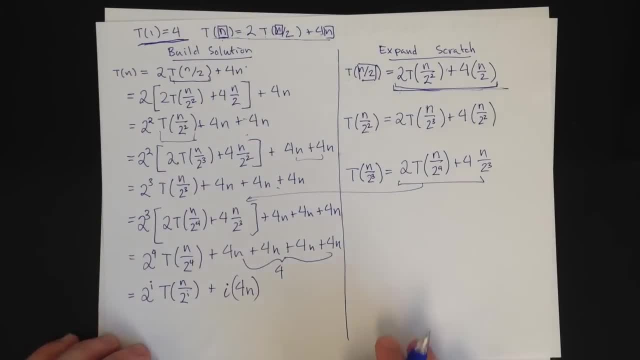 that becomes 4, and there's nothing left to expand. So the way to answer this is to say: well, what's in here? 1.. So what I need to get is a 1 in here, which means that n divided by 2 to the i. 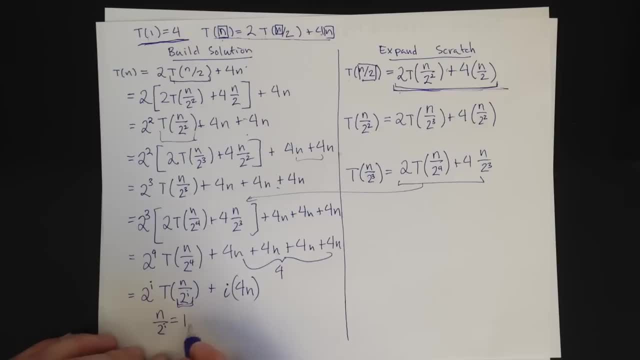 needs to equal 1.. If I multiply both sides of this equation by 2 to the i, I get n is equal to 2 to the i And then, remembering your logarithm identities, this means that the log base 2 of n is equal to i. 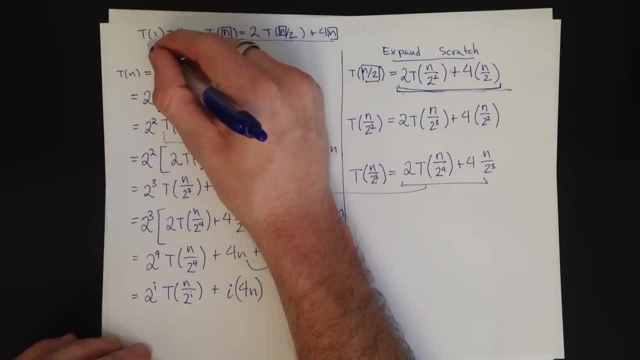 before I simplify it. How many times would I do this before I stop? Which is asking: how many times do I do this before I get down to a base case? That is, when I stop Because, notice, if I get to t of 1,. 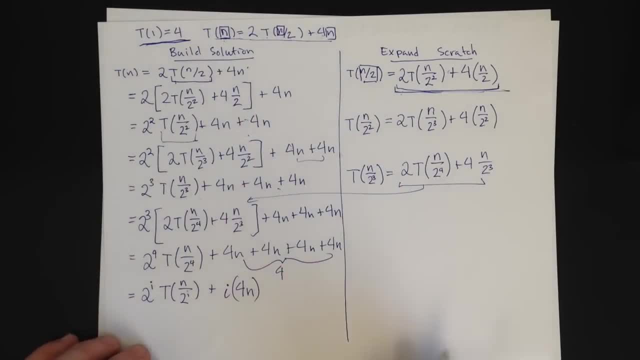 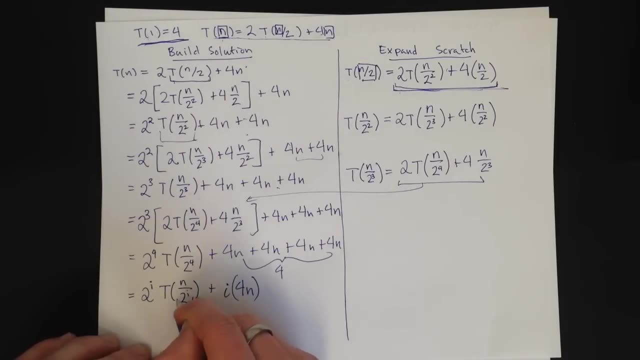 that becomes 4, and there's nothing left to expand. So the way to answer this is to say: well, what's in here? 1.. So what I need to get is a 1 in here, which means that n divided by 2 to the i. 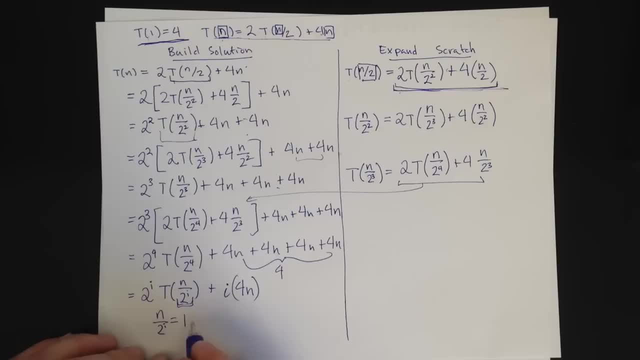 needs to equal 1.. If I multiply both sides of this equation by 2 to the i, I get n is equal to 2 to the i And then, remembering your logarithm identities, this means that the log base 2 of n. 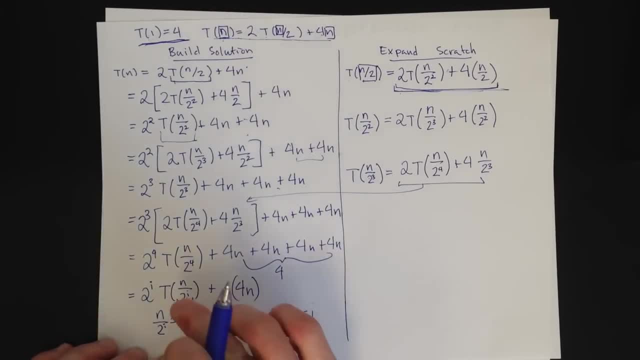 is equal to i, So that is the value for i, at which this becomes t of 1.. And so now I can just plug in this equation for i into my generalized equation. I'm going to do that over here, And what I get is: 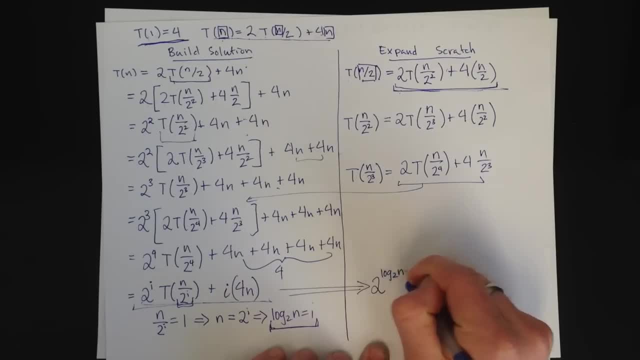 2 to the log base 2 of n. So I plug that in Times t of 1.. Because I've already shown you that that's how I got this i. That was the i that that turns into 1.. Plus log 2n times 4n. 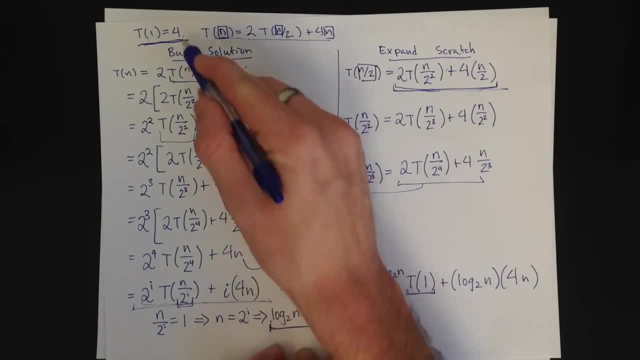 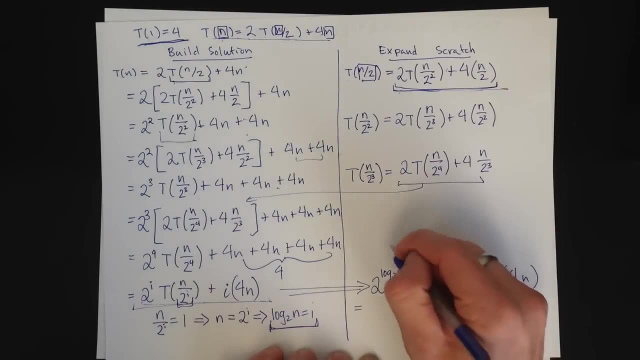 So far, so good. Well, we know what t of 1 is. t of 1 is 4.. So that's going to become a 4.. And then the question is: what is this? 2 log base. 2 of n. 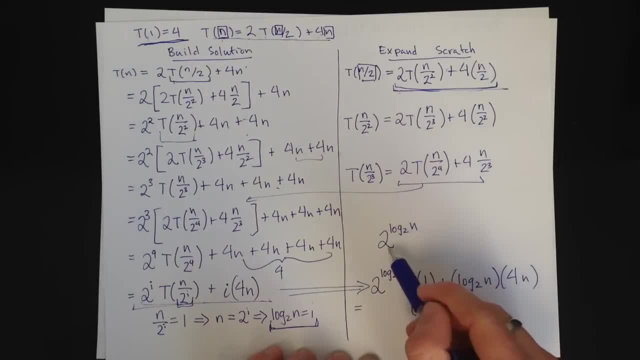 Well, there's an identity that you need to remember, Which is when I have something to the log of something else, I can always swap. So this becomes n to the log base 2 of 2.. How many times do I have to raise 2? 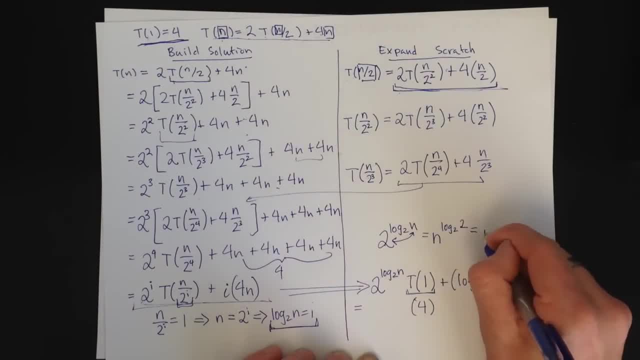 to a power to get 2?? That is 1.. So this is equal to n. So what I get this becomes n plus 4n log base 2 of n And writing this a little more naturally, is 4n log base 2 of n. 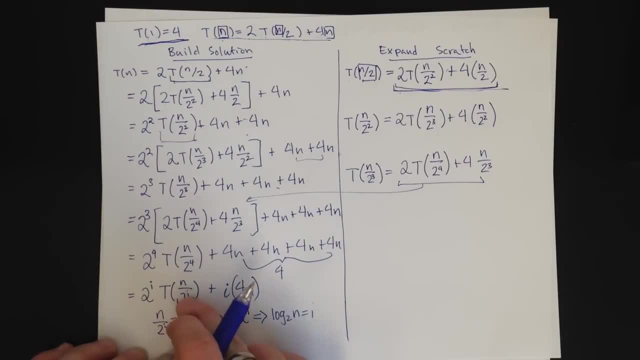 So that is the value for i, at which this becomes t of 1.. And so now I can just plug in this equation for i into my generalized equation. I'm going to do that over here, And what I get is 2 to the log base, 2 of n. 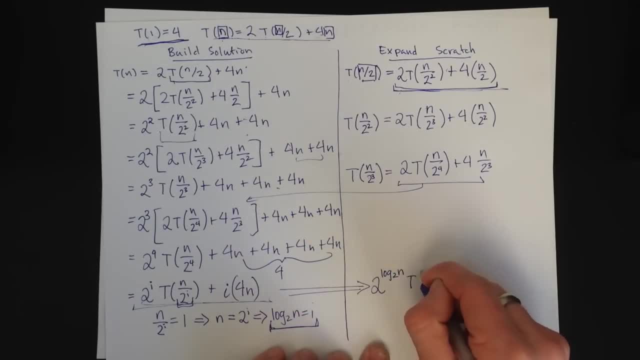 So I plug that in Times t of 1. Because I've already shown you that that's how I got this i. That was the i that that turns into 1.. Plus log 2n times 4n. So far, so good. 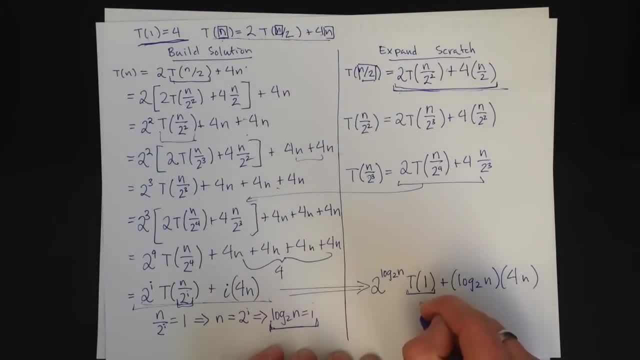 Well, we know what t of 1 is. t of 1 is 4.. So that's going to become a 4.. And then the question is: what is this? 2 log base, 2 of n. Well, there is an identity that you need to remember.